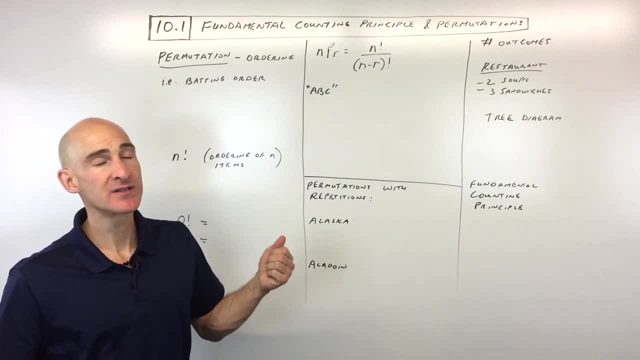 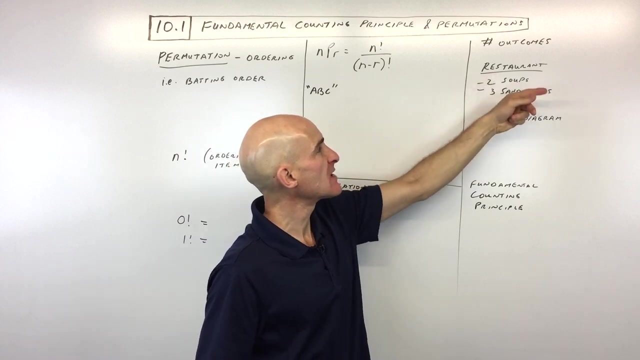 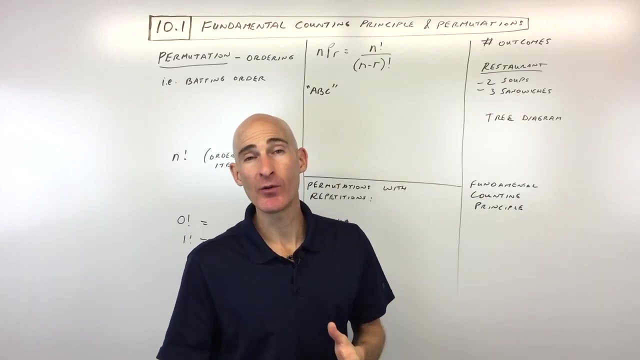 Okay, chapter 10.. We're going to start off with 10.1, talking about permutations as well as the fundamental counting principle, And what this is aimed at is how to find out the number of outcomes that are possible. So let's start off with talking about a simple example. Just say, for example, you go to a restaurant and there's two soups- you can choose one of the two soups, And there's three sandwiches and you can choose one sandwich. How many different like lunches could you have with one soup and one sandwich? Well, we can. 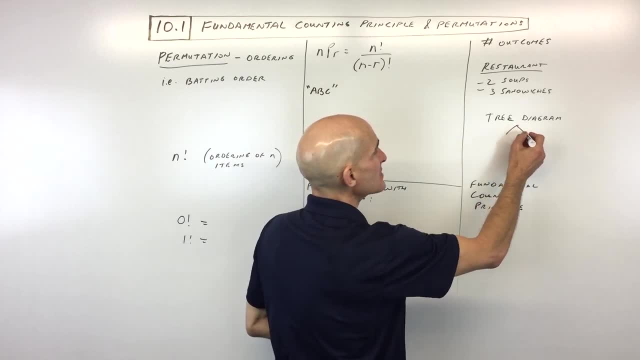 diagram this using a tree diagram by basically saying: okay, you could choose soup number one, or you could choose soup number two, and then you could choose one of three sandwiches. And so if you look at these end points here, you can see there's six possible routes that you could. 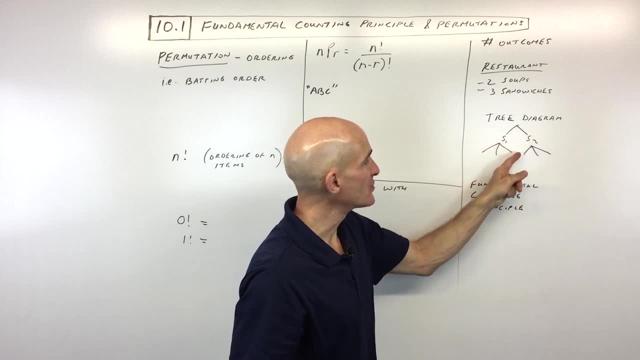 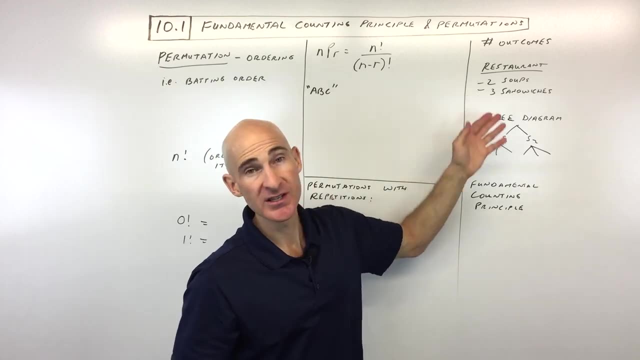 take. you could go down this route or down this route or down this route, But you can see there's going to be an end result of six different possible outcomes. Now, when there's a lot more choices, the tree diagram would get a lot larger and it'd be a lot harder to calculate. 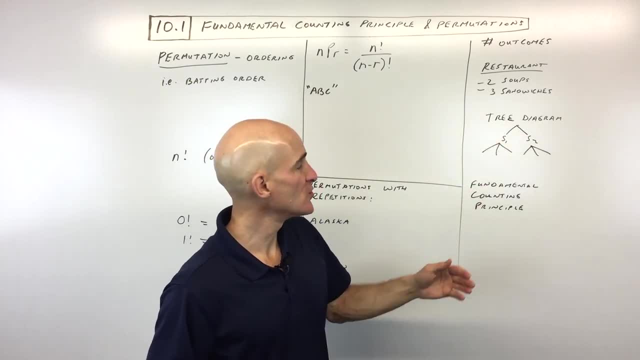 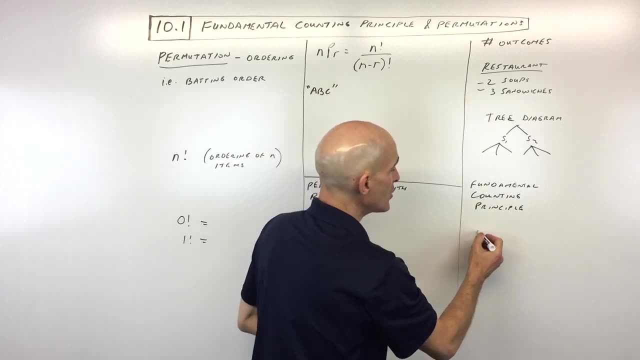 By you know, making this big tree diagram. So an easier way to do it is to use the fundamental counting principle, And the way this works is you look at how many choices there are in each category. So, for example, there's two sandwiches possible. you're just going to pick one of the. 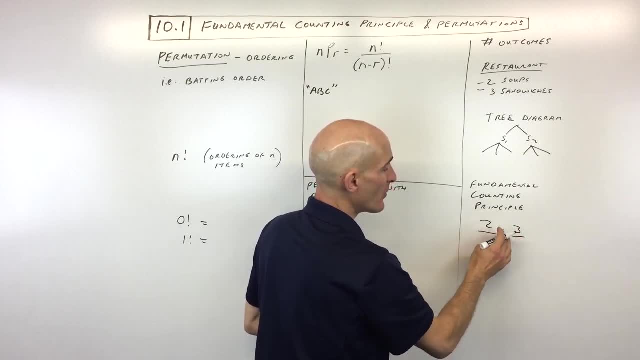 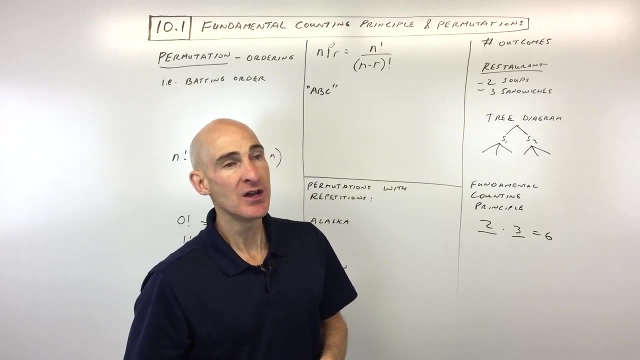 two, there's three sandwiches. you're going to just choose one of the three. So if you multiply two times three, you can see you're getting the same six outcomes we had, as we saw in the tree diagram. So that's a nice technique. fundamental counting principle for finding the number of. 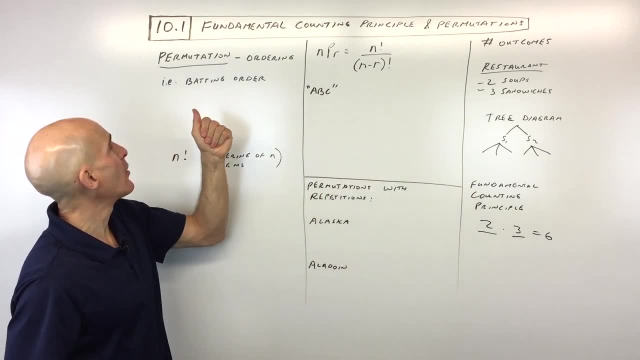 outcomes. Let's look at another type of problem That you're going to encounter, And that's when you're talking about a permutation. A permutation is basically an ordering of items. So you say: well, you know, how many ways could I, you know? 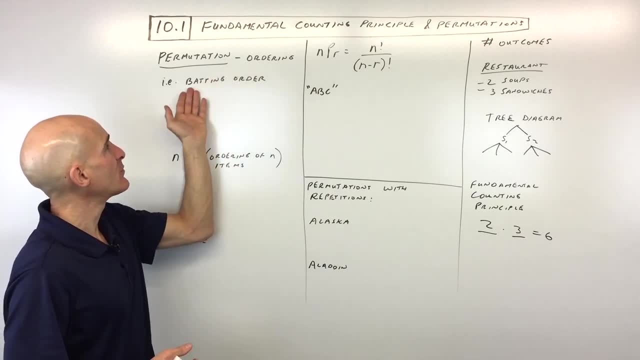 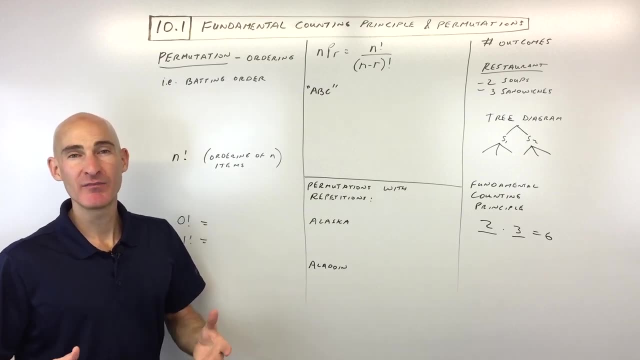 order n items. Okay, An example would be like: say: for example, you had a batting order, So there's nine basically batters in a baseball game, right in a batting order. And so you say: well, how many ways you know, could you rearrange that batting order so that maybe the catcher 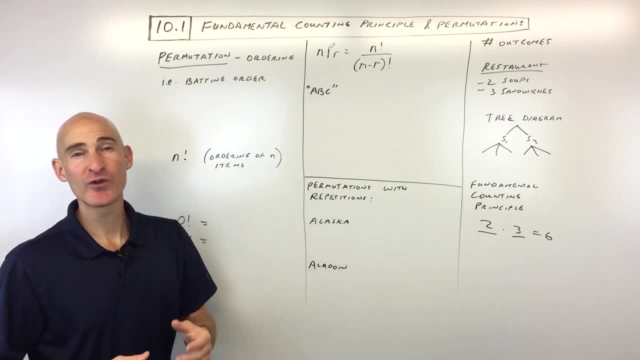 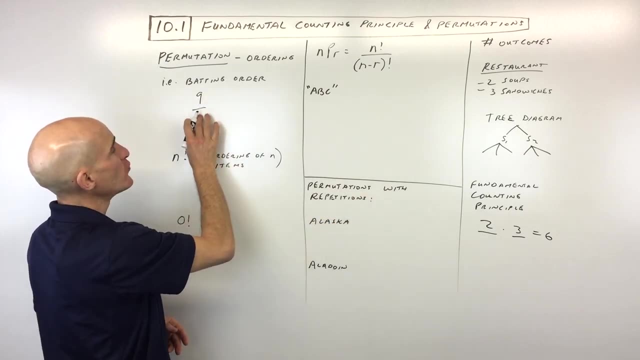 bats first, or maybe the pitcher bats second, or you know you want to rearrange all of those different players. So one way to do it is just to use the fundamental counting principle. You could say: well, there's nine choices for who bats first. Once you pick that person, that bats. 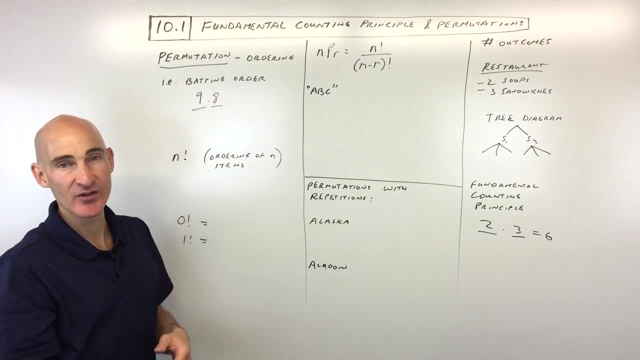 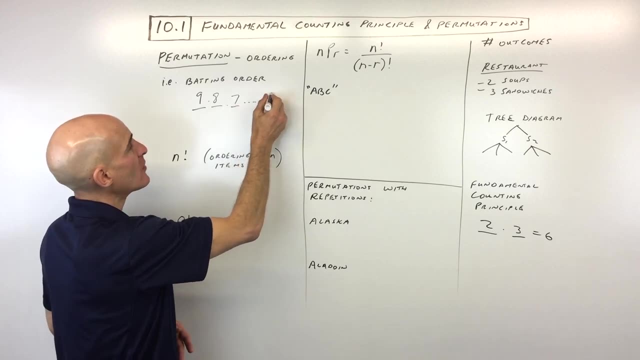 first, then there's going to be nine- I'm sorry, eight- choices for who bats. you know that. second position: Once you pick those two batters, there's going to be seven people left. You're going to choose one of those to bat third, all the way down to one. And if you multiply those together, 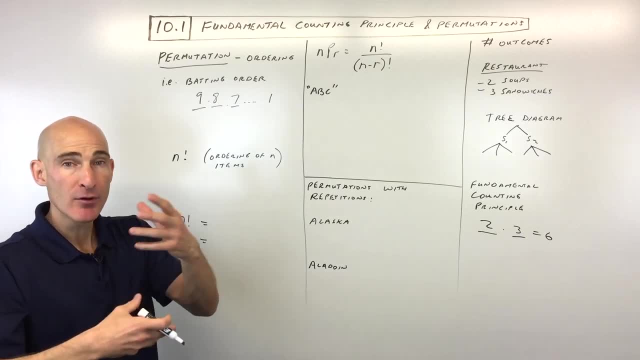 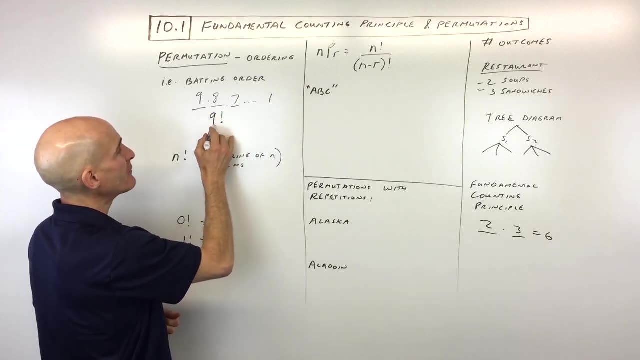 that's going to give you the total number of, you know, batting orders or possible permutations or orderings of those players. So what I'm going to represent this is with a factorial, nine factorial, And I'm going to show you where this is on your calculator in just a moment. But the this exclamation point just 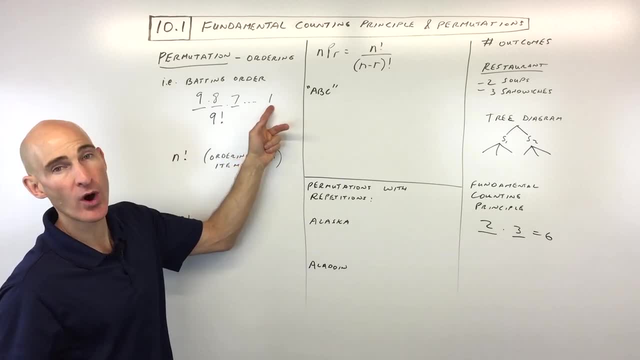 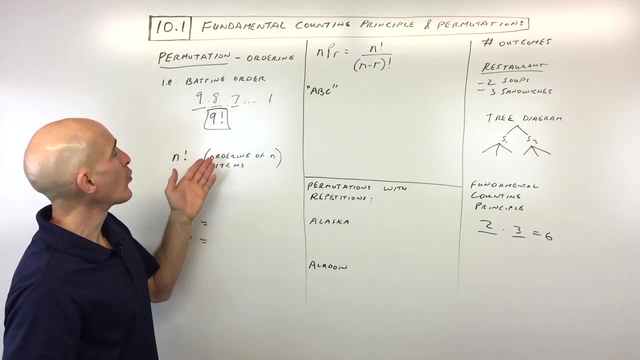 represents taking this number nine and multiplying all the way down to one. So it's just like kind of like a shorthand way of describing that So fundamental counting principle. or you can use this formula: n- factorial, and that's just an ordering of n distinct or unique or different. 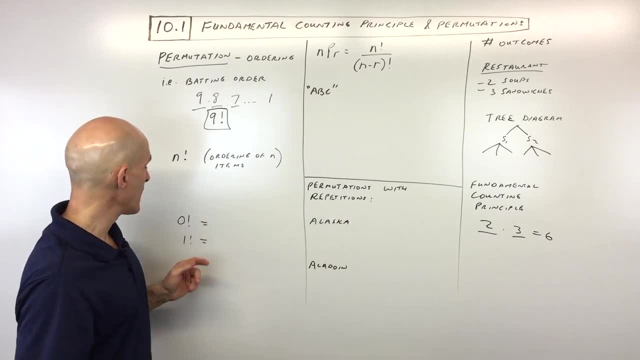 items. How many ways could you rearrange them? So n factorial. now, one thing to realize is that zero factorial. you just have to memorize this. one it's equal to one. one factorial is one, And then after that, two factorial would be like two times one, three. 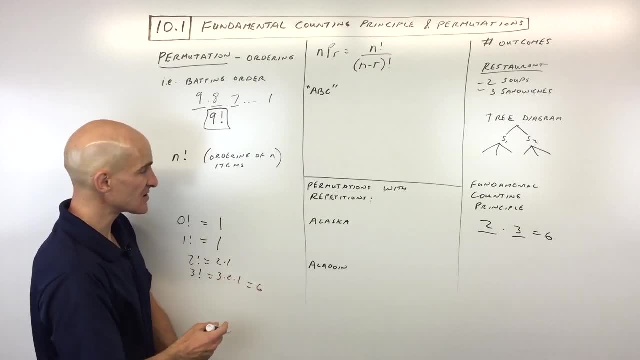 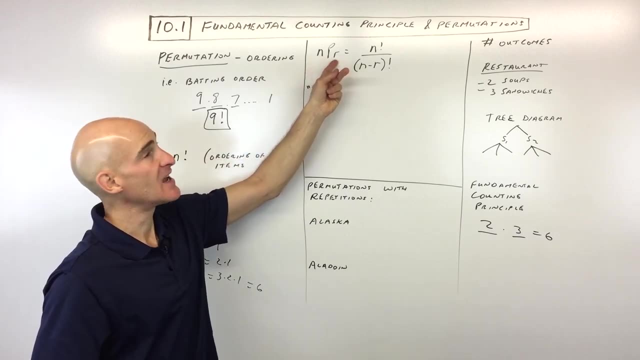 factorial three times, two times one. you know which is six, etc. Now another concept we want to talk about here are permutations of n items taken r at a time. So what that means is say, for example, you had the letters ABC And you said, Well, I just want to choose two of those. 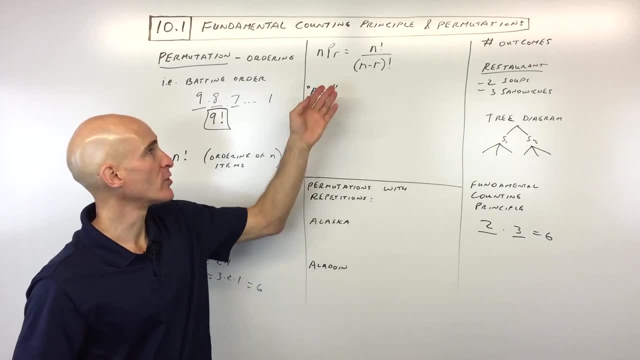 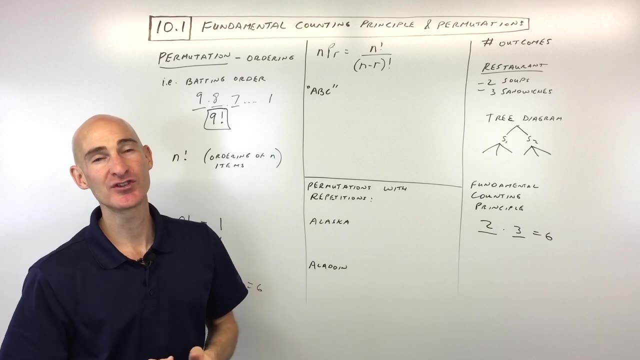 letters. So you can see that the order is important. you can see the order is important where the order matters. the order is important when you're talking about a permutation because if you switch them, you know, say, for example, you have, like a president, a vice president. if you switch those, 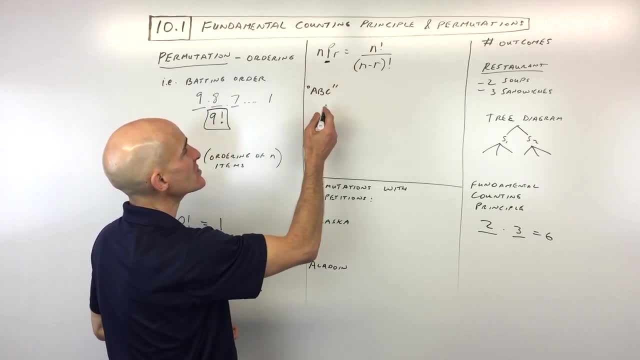 two people, they're going to have two different jobs, right. So it's going to be important to order when you're talking about permutations. But let's just see if we can write out the possibilities here. you could have A and B. you could have B and A. okay, that's a different permutation. you. 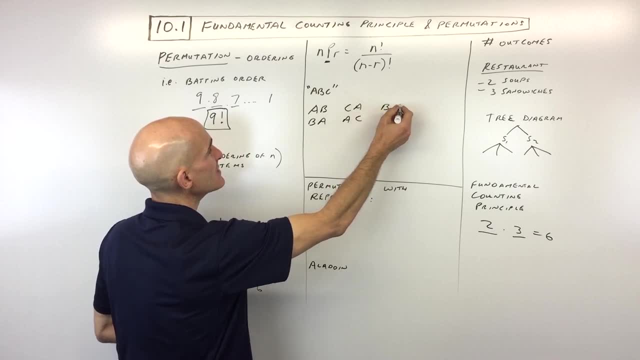 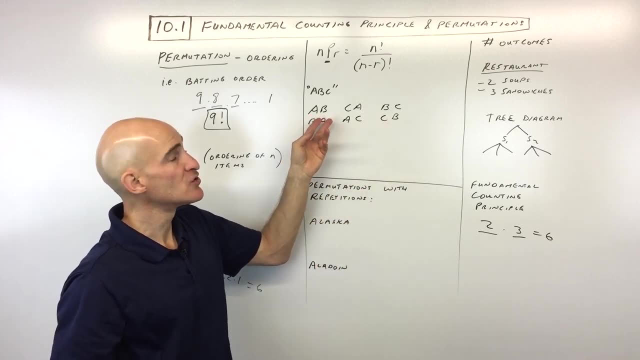 could have C and A, you could have A and C, you could have B and C, or you could have C and B. So different permutations of the two letters out of the three possible. So you could either write them all out and count them up, but as you get working, 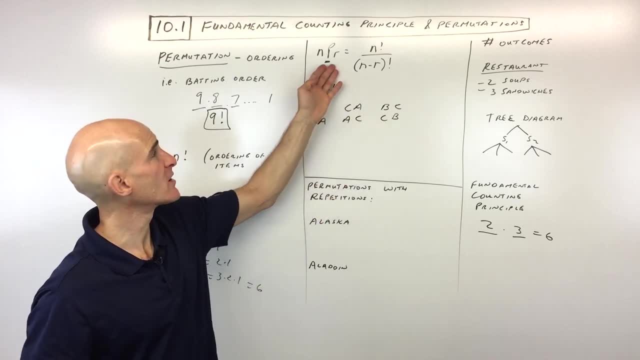 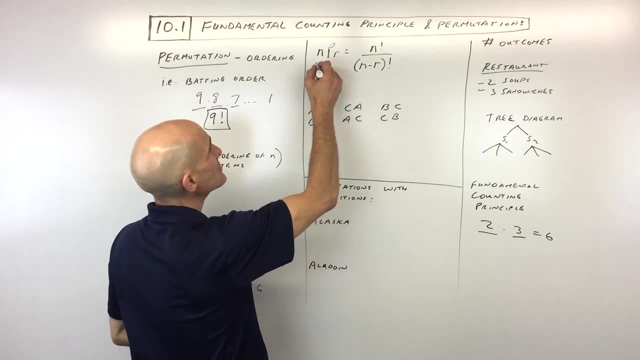 with larger items, it's going to be very difficult to do this. So that's where this formula comes. in NPR it equals N factorial over N minus R factorial. So for this example, N is three, because we have three items- A, B or C- and we're 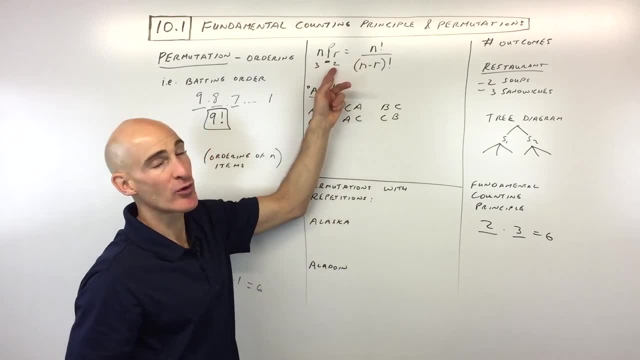 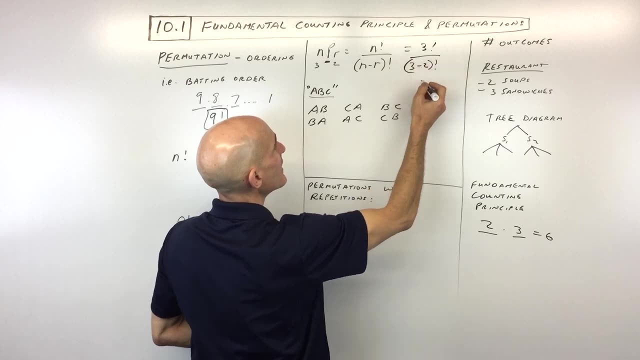 picking. okay, you can think of you're picking two of them where the order matters. So we can see here this is going to be three factorial and then three minus two factorial. Well, three factorial is really like three times two times one, and three minus two is just one factorial which is just one. So you can. 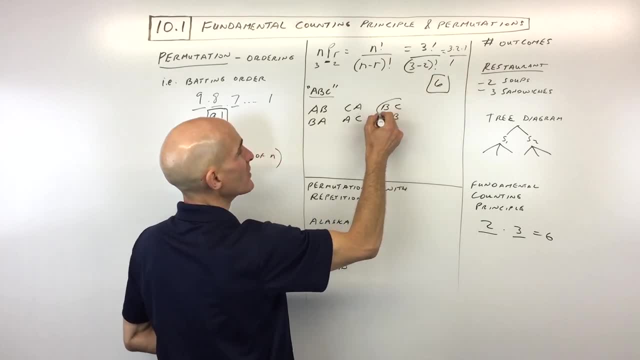 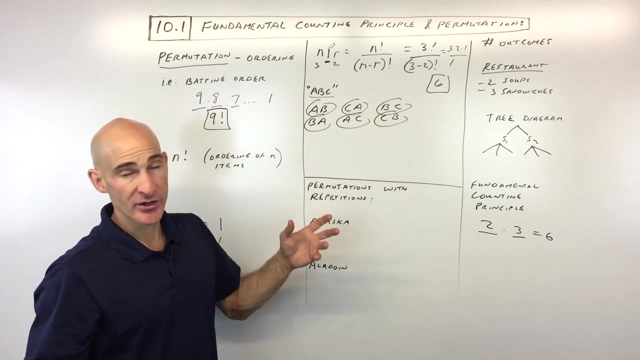 see, this is six divided by one, which is six, and that's the same result that we got here: the six different ways of picking two items out of three. So the last concept I want to talk about before we get into some examples that you can. 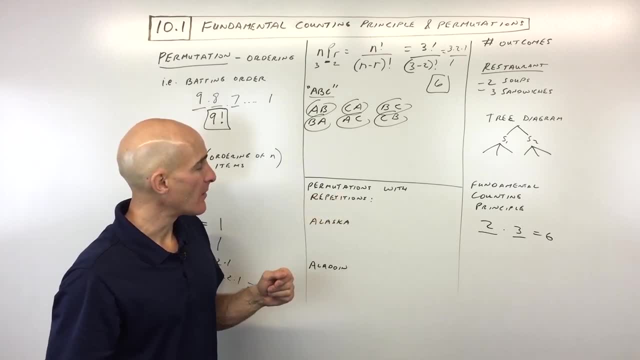 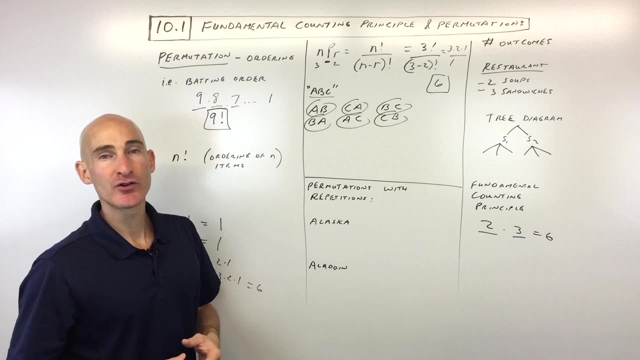 practice are talking about permutations with regular items. So we're going to talk about permutations with regular items, repetitions. Now what does this mean? Well, see over here we talked about N factorial. This is an ordering of N distinct or different or unique items. 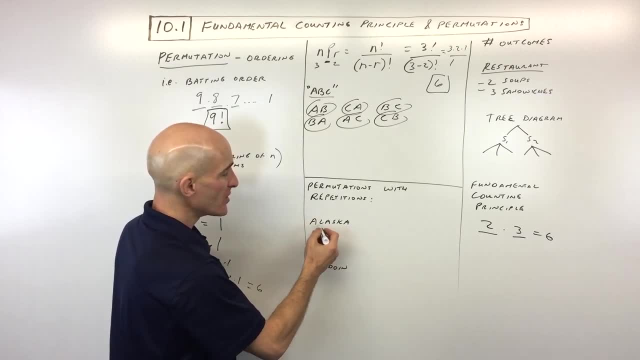 But say, for example, you want to see like, how many ways could you rearrange the letters in the word Alaska? Okay, so you can see there's one, two, three, four, five, six letters. So normally we would say there's six factorial ways of you know. 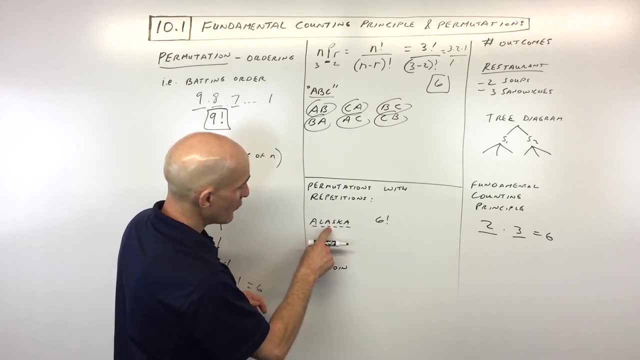 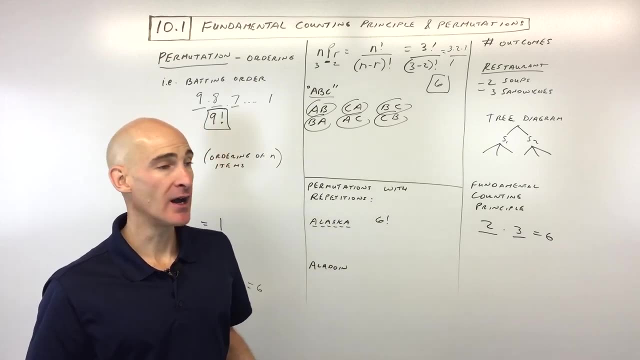 arranging these six items. The only problem is is that if I put this A over here and this A over here and this A over here, it would still look like the word Alaska, So it's not really like a distinct or a different way of, you know, representing. 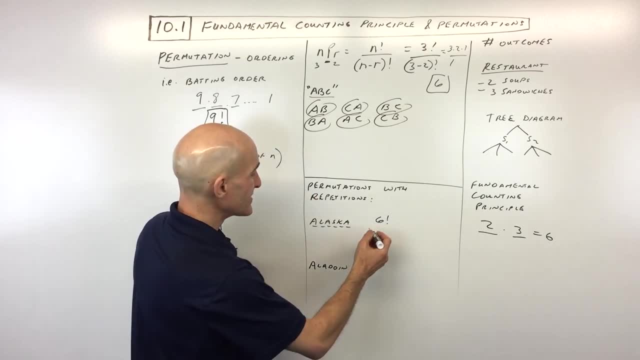 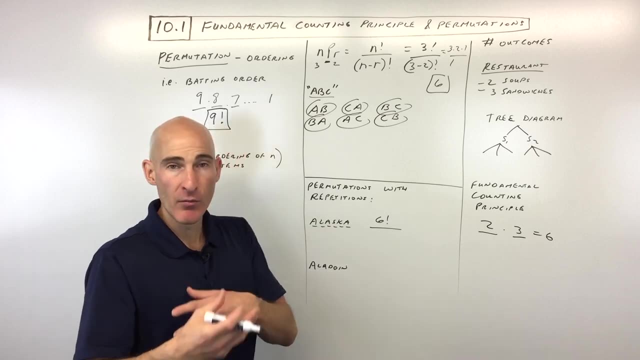 those letters It would look the same. So if we want to look at the different ways of representing these six letters, different orderings, the different permutations, we have to divide out the multiplicities or the duplicates, or the triplicates. So the way we would do that is, if we've got three A's, we're going to 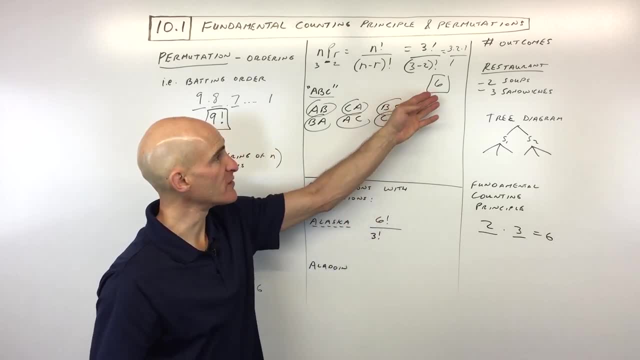 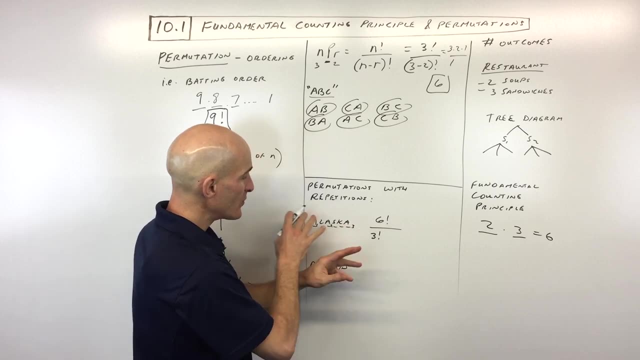 divide by three factorial- Remember, three factorial from this problem was three times two times one, which is six. So there would actually be like if we were to label this as A1.. A2.. A3. There will be six different ways to arrange these three A's, but it would still look. 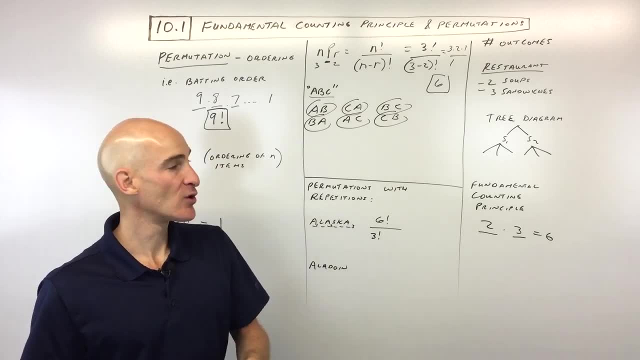 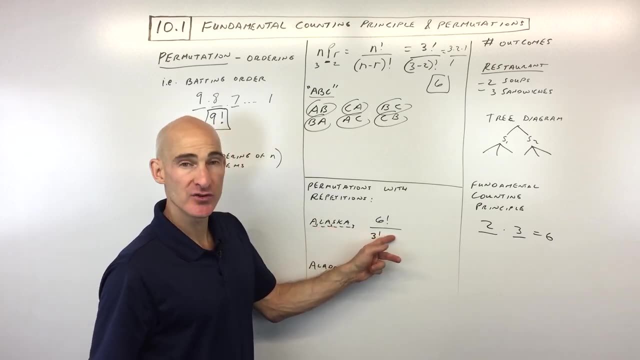 like the word Alaska. So we don't want to, you know, count that six times. We only want to count that word as Alaska once. Also, are there any other duplicates? If there were any other duplicates, we would divide by those other. let's say there: 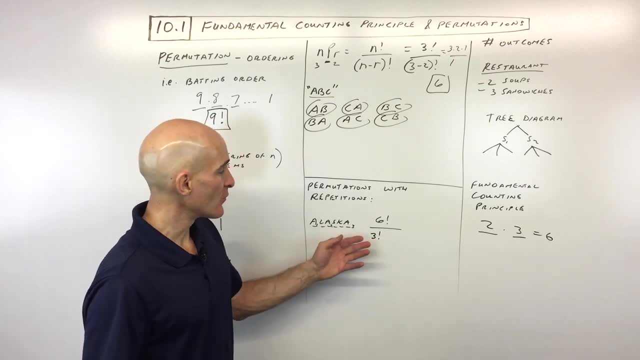 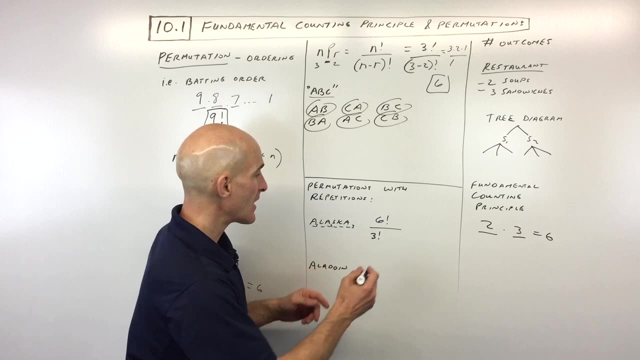 was like two L's, I would divide by two factorial, etc. So from here you can simplify. but don't make this mistake: Six factorial divided by three factorial does not equal two factorial. So you just have to write this out. It's going to be six times two factorial. 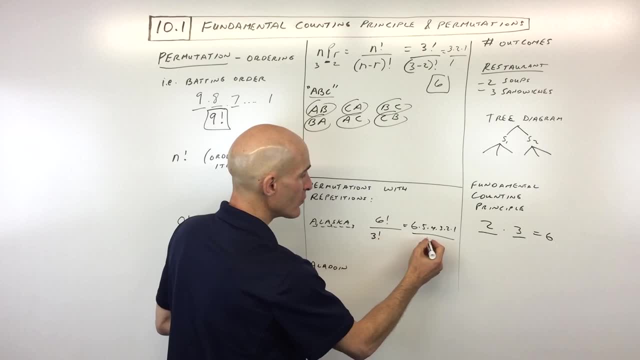 five times four times three times two times one over three, factorial, which is three times two times one. notice the three, two and one. cancel. we just have: uh, six times five is thirty times four is a hundred and twenty different orderings of the letters in the word alaska that are different. 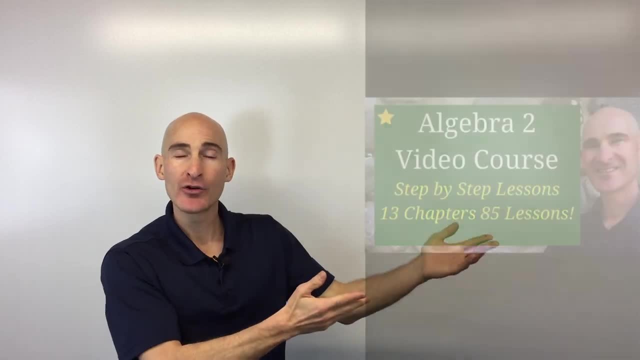 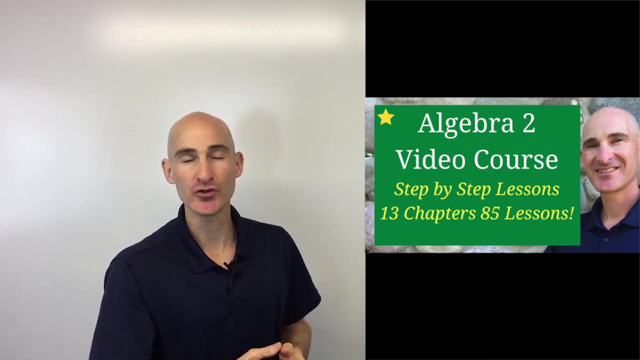 now let's look at another example to learn algebra two. check out my learn algebra two video course for sale, where we go through 85 video lessons that take you step by step by step through algebra 2.. we go through the important formulas, concepts, as well as. 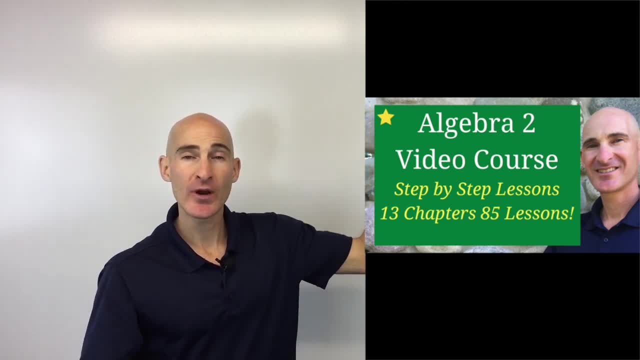 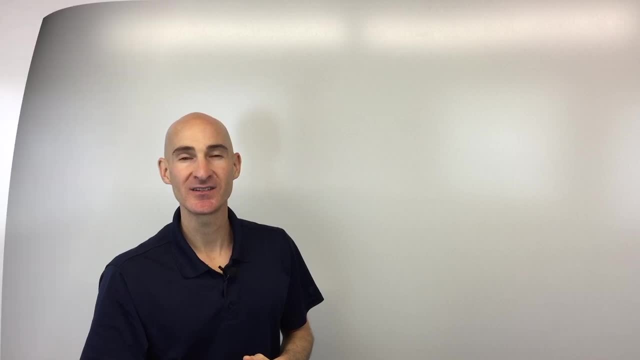 numerous examples to help you master algebra. 2. click the interactive card or the link in the description below to go over and check out some of the free lessons. otherwise let's get back into this current lesson, different. now let's look at another example. say we have aladdin right. 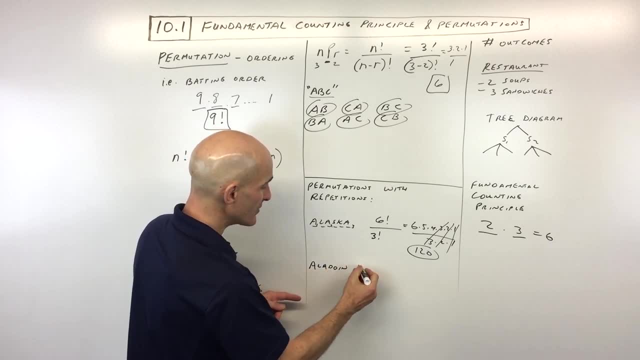 so, laden, we have one, two, three, four, five, six, seven. so there's going to be seven factorial ways of arranging those letters. but because we have two a's, we're going to divide by two factorial. and we also have 2d, we're going to divide by 2 factorial again. this does not equal 4 factorial, you just have to just. 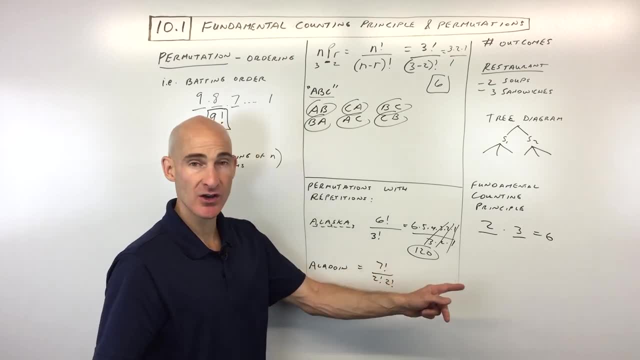 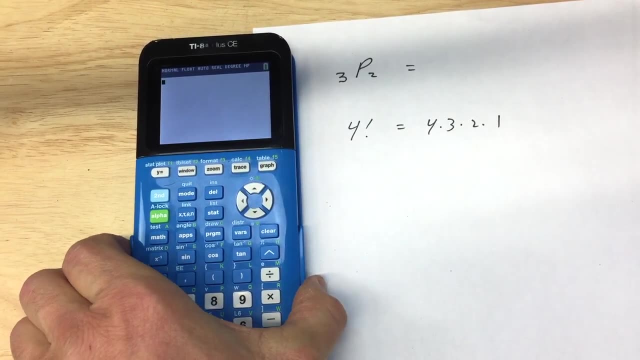 do them separately. so 2 times 1, 2 times 1, and then 7, 6, all the way down to 1 and you can reduce. hey, I want to show you on the TI 84 where some of these key functions are, these key buttons. so 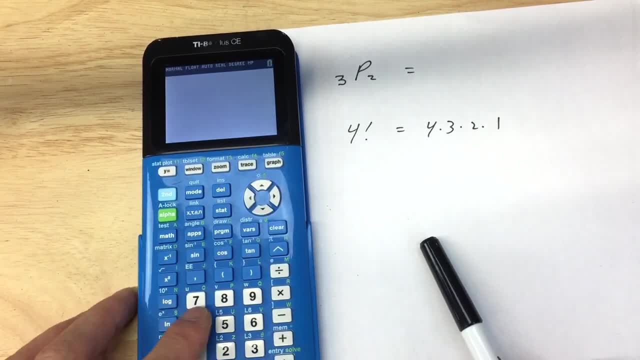 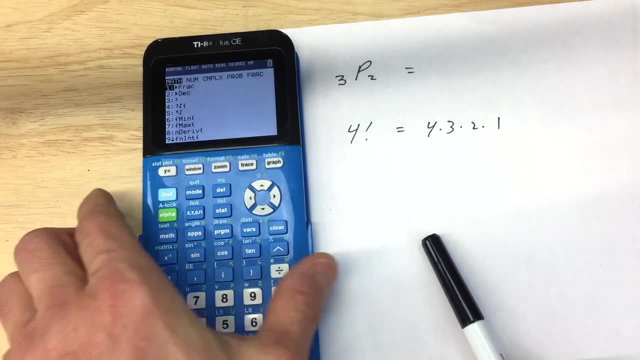 let's go ahead and calculate 4 factorial. so what you would do is you would type in 4 and you would go over here to math. it's the 1, 2, 3, 4th key down here on the left. so math. and if you take a look, 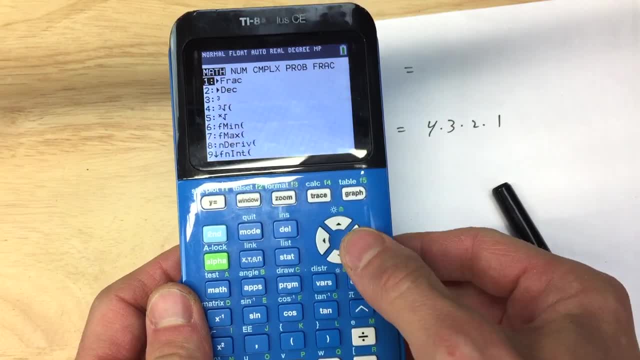 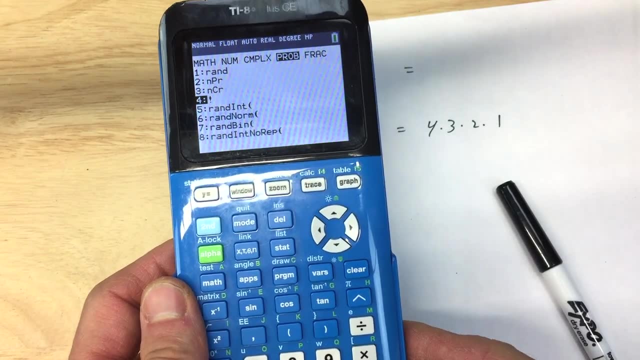 over here where it says probability pure. OB, you just want to arrow to the right probability and then arrow down to the number 4. it looks like an exclamation point. so that's your factorial notice. above it, you've got your combinations, which we're going to talk about in a future lesson, and the 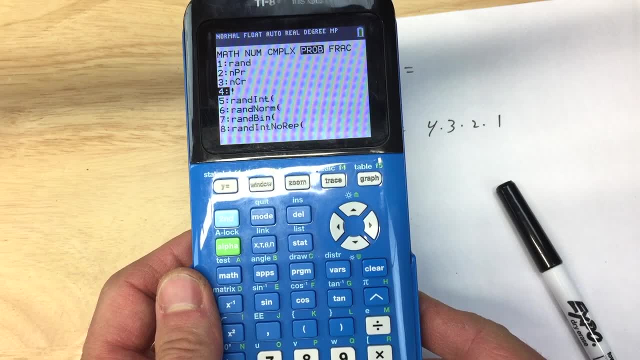 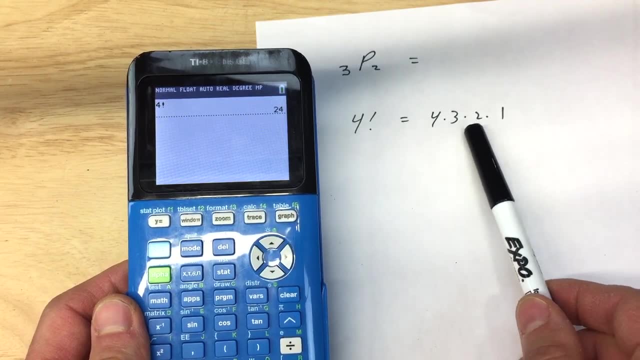 permutations: NPR. but for right now let's just go ahead and press the number 4 factorial. so 4 factorial is 24 and it makes sense over here you can see: 4 times 3 times 2 times 1, 4 times 3 is 12. 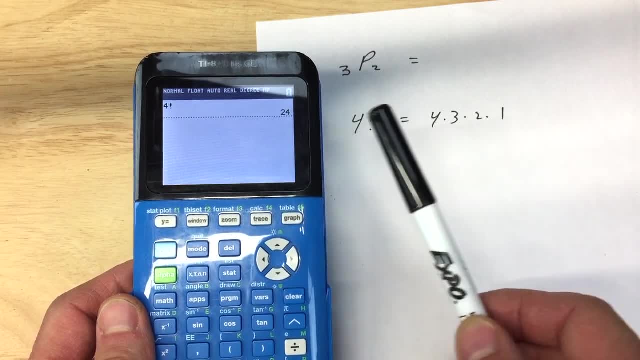 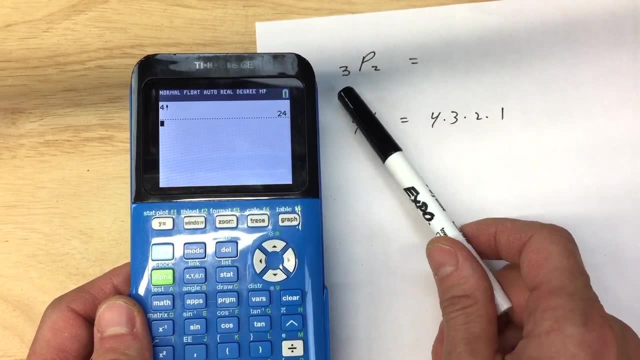 times 2 is 24, times 1 is still 24. so just a shortcut here. you can use your calculator for some of these ones where it's a larger than 4. you know larger numbers. let's go ahead and look at number 3: permutation. 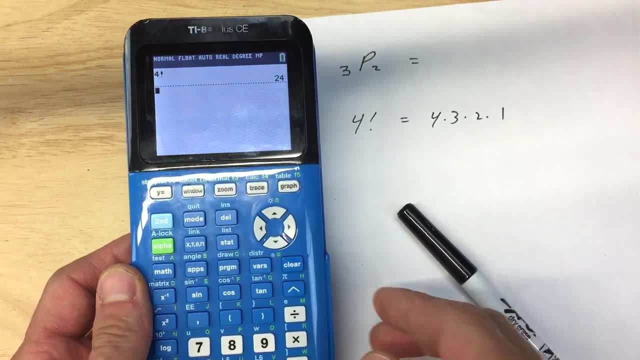 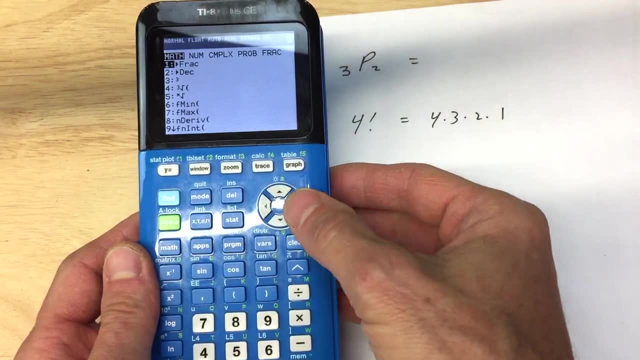 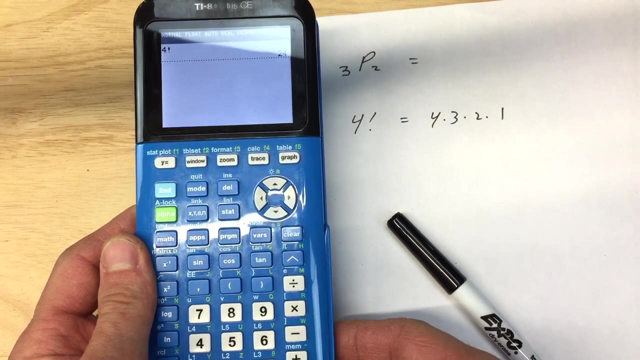 2, so out of 3 items you're picking 2, where the order matters. we did an example like that in the lesson, but what you would do is you would go ahead and type in 3, go over to math again and you want to air over to probability, down to number 2, permutations and 3, P 2, and press ENTER in the 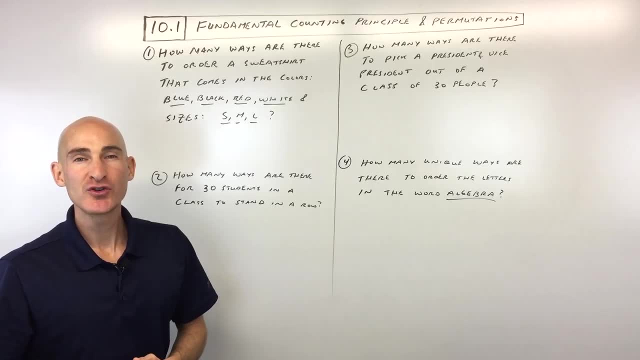 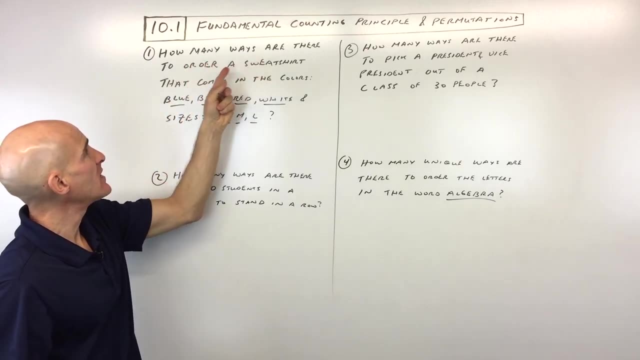 lower right hand corner and you can see it comes out to 6. okay, here's your opportunity to practice, so go ahead and pause the video and do each problem on your own. we'll go through them together. number one: it says how many ways are there to order a. 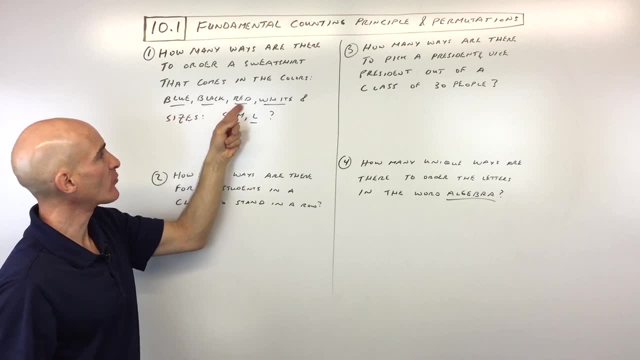 sweatshirt that comes in the following colors: blue, black, red and white. and then it comes in the following sizes: small, medium or large. so how would you do that problem? you're trying to figure out how many different sweatshirts that are possible. to order different sweatshirts, right. 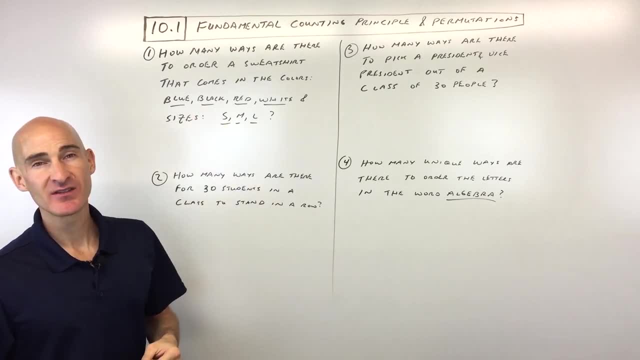 given the four colors and the three sizes. well, if I was going to do this problem, I'd use the fundamental counting principle and I'd use the fundamental counting principle, and I'd use the fundamental counting principle and I'd say 4 times 3. there's 12 different possible outcomes. the 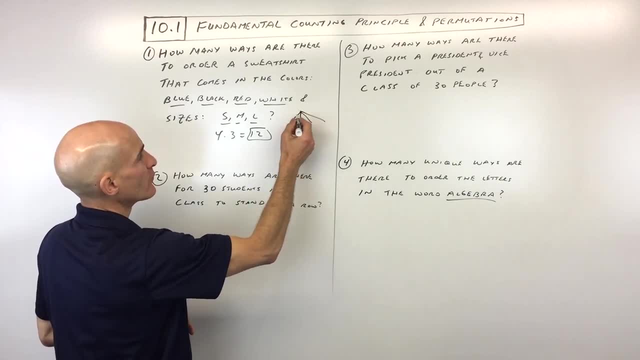 other option that you can do is you can make a tree diagram so you can go to four different colors and then, once you pick that particular color, you have three sizes, so you can make a tree diagram that looks like that, and if you count the ends here, you're going to see that. 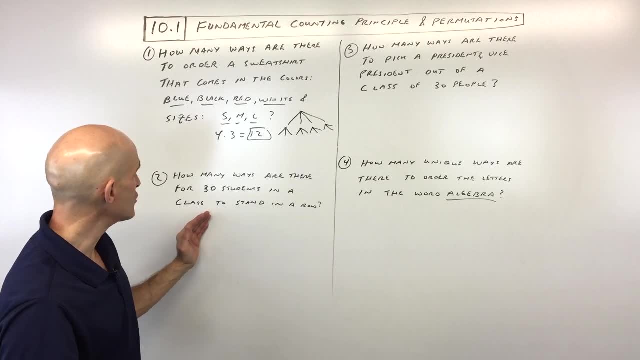 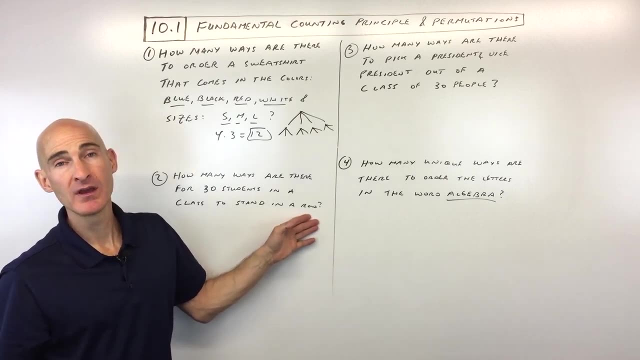 there's 12, so answers 12 for number one. so for number two, try this one. how many ways are there for 30 students in a class to stand in a row? so we can kind of visualize that there's 30 people in a whole class. how many ways could they stand in a straight line in a row? how would you do that one? 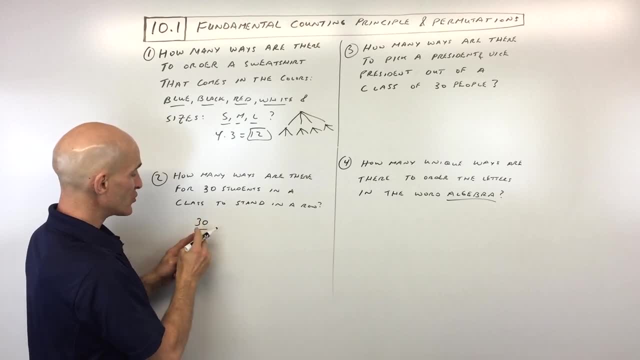 well, this one. you could diagram it out if you want. you can say: there's 30 choices for who stands furthest to the left here. once you pick that person to stand furthest to the left, there's 29 people to choose from. to pick that person to stand second for this to the left all. 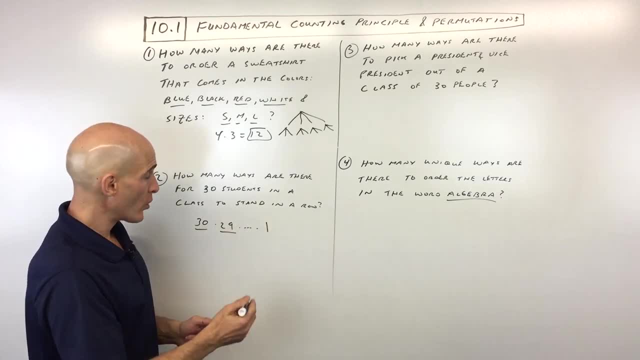 the way down to one. you would multiply those together or you could use 30 factorial. this is just using the formula n factorial. that's a way of how many ways can you arrange n items and then look robust to this. you can do asti different items and so that's it: 30 factorial. you can do this on your. 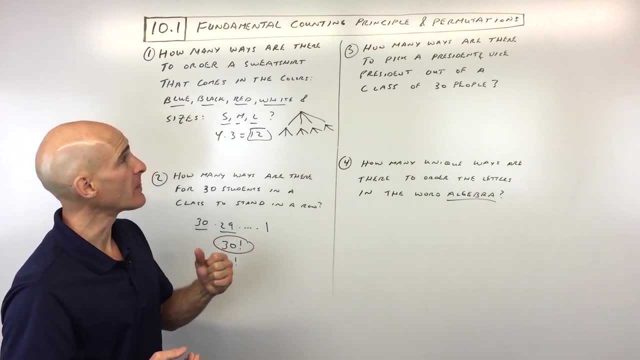 calculators can be quite a large number. okay, how about number three? it says: how many ways are there to pick a president and a vice president out of a class of 30 people? okay, so now here you can see. the order is important because if you switch those two positions- president, vice president- you know the two students. 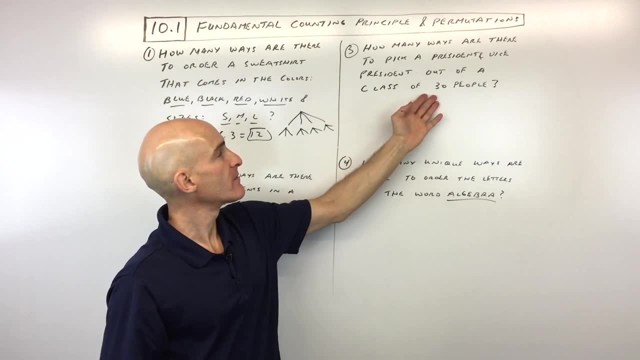 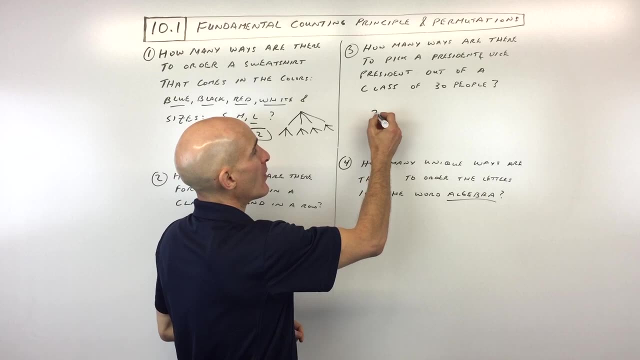 would have a different job, but how would you do that one? so what do you think? well, if I was going to do it, I recognize that it's a permutation, it's an ordering right, but what we have is 30 people and we're picking two where the order? 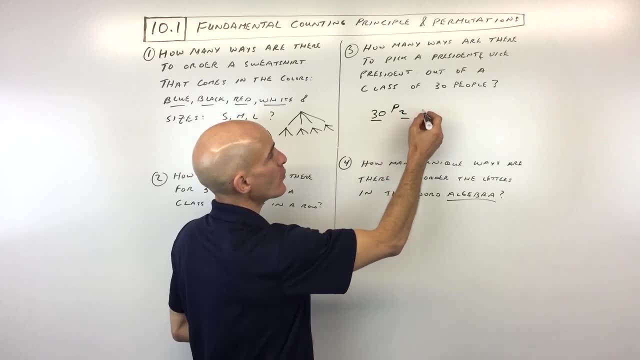 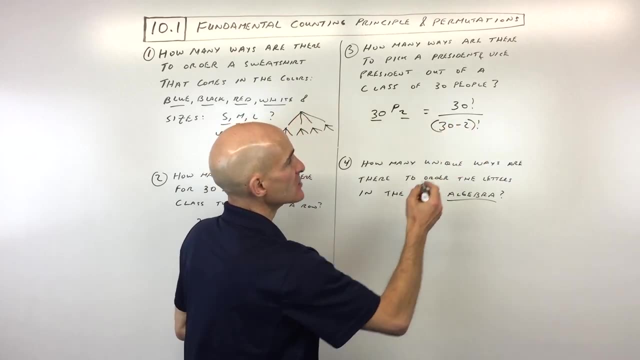 matters. so we've got 30 P 2. now remember our formula: it's n factorial over n minus R factorial, and so if you go ahead and expand this out, you can see this is going to be 30 times 29 times 28, all the way down to 1. okay, 30 minus 2 is 28. 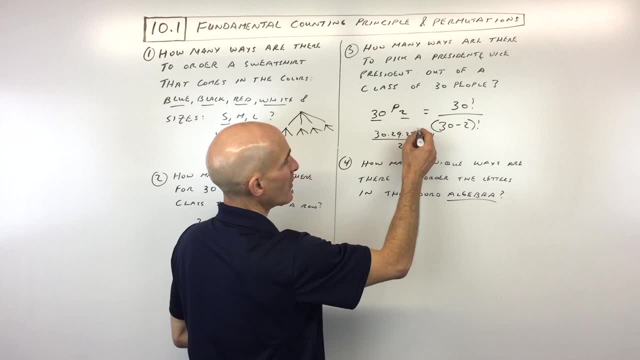 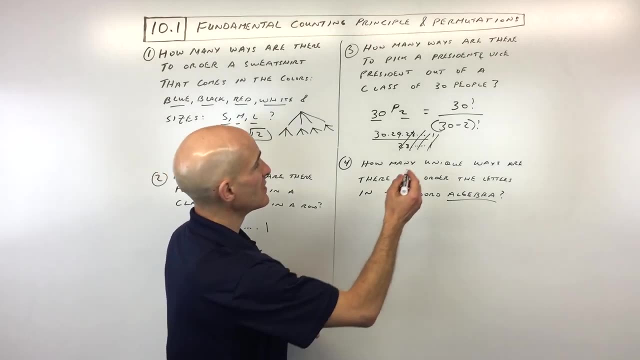 factorial, which is 28, 27, 26, all the way down, multiplying all the way down to 1, those cancel. so it's really just going to be 30 times 29 and if we do that on the calculator you can see that's going to be 870 different ways of picking a. 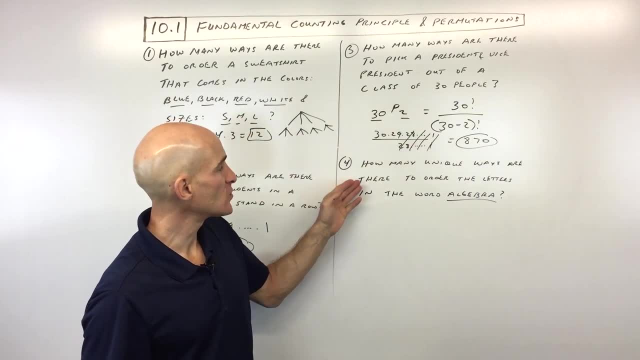 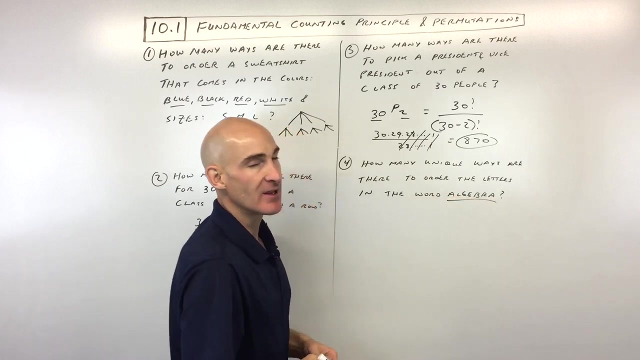 president and a vice president. okay, last problem, see if you can do this one. how many unique ways are there to order the letters in the word algebra, right? so this is like an algebra 2 type question. so let's see it's very appropriate here. so what do you think? there's 1, 2, 3, 4, 5, 6, 7 letters. notice that there's some. 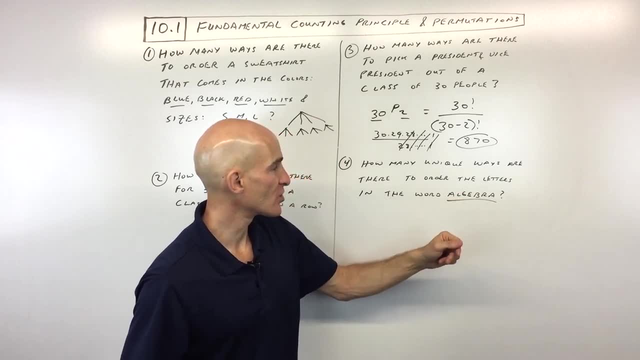 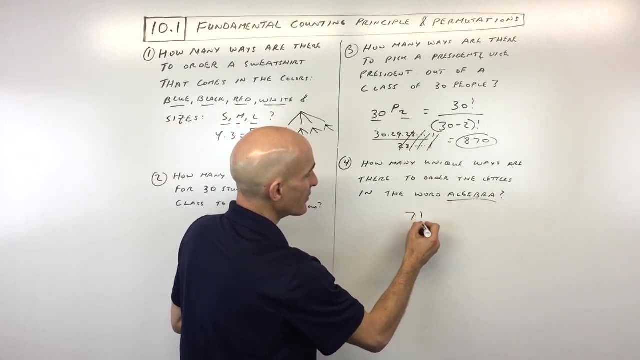 repetition. here we've got two a's. all the other ones just occur once. so how do you, how would you do that one? well, if I was going to do it, I would say: okay, there's, we said seven letters and there's two a's, so there's actually two different. 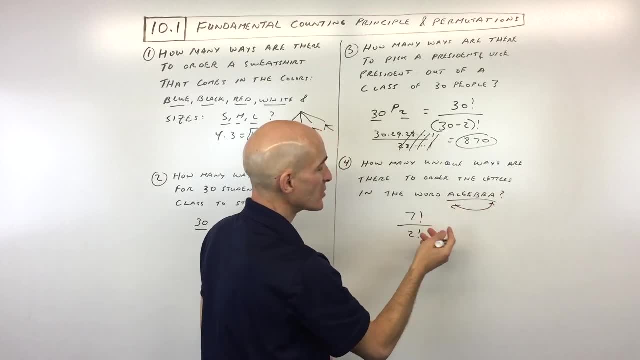 ways of you know, if I interchange these two a's, it would still look like the word algebra. so we want to divide out those multiplicities, those duplicates, and so if we simplify, this is going to be 7 times 6 times 5 times, 4 times 3.